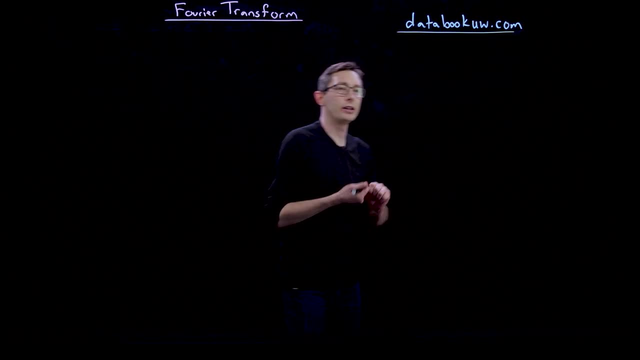 And so how do I want to think about this? So I'm going to have- I guess I should write down some problems. So the heat equation we're going to say is: ut equals some positive constant. I'm going to call this alpha squared because I don't want to have like negative heat diffusion. 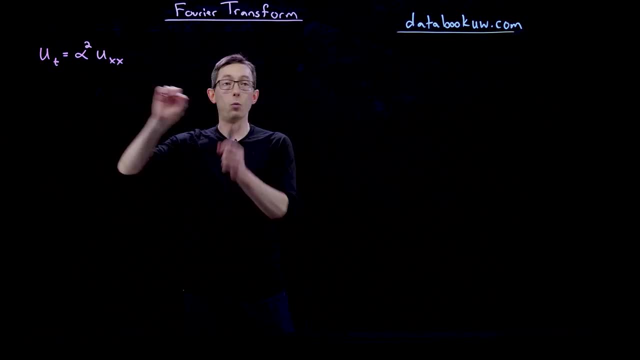 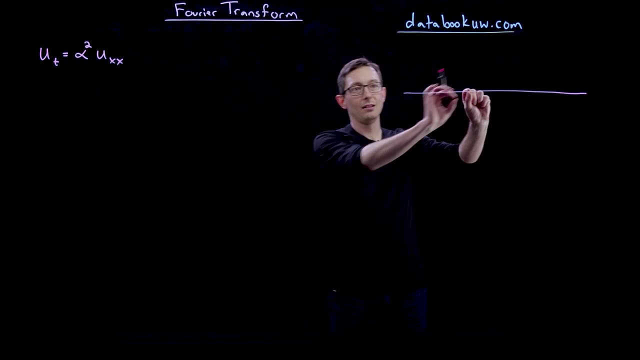 uxx. okay, So this is a 1d heat equation. This is the 1d heat equation and the way you can think about this is that you have kind of an infinite, maybe like a thin piece of metal, a 1d piece of metal with some initial heat distribution. 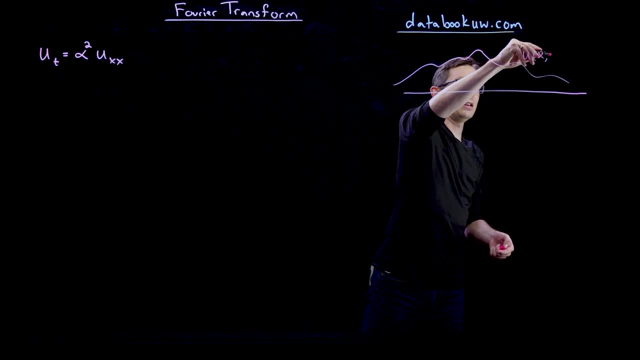 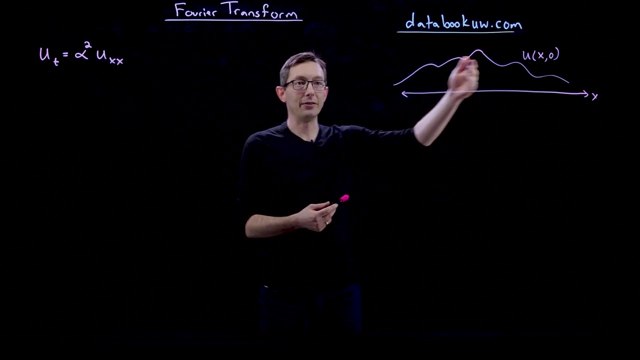 that we're going to call u at x at time zero, u of all of space at time zero is my initial temperature distribution. okay, And as x goes to plus and minus infinity, this thing is going to have to die off to zero, otherwise this would have infinity. So we're going to have a 1d heat equation. 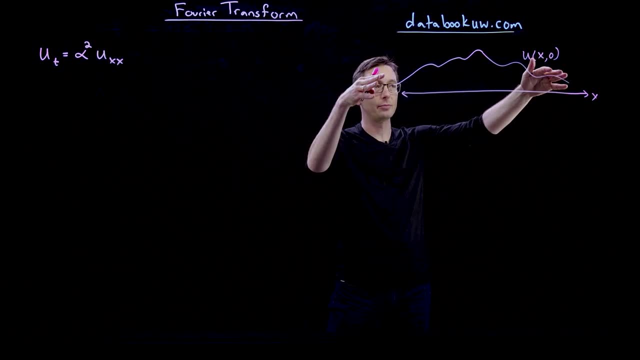 infinite heat energy, which is non-physical. okay, So I have some initial temperature distribution. I'm assuming that that temperature eventually will die out to zero, at plus and minus infinity, so that I don't have infinite temperature, infinite heat energy in this thin 1d piece of metal. 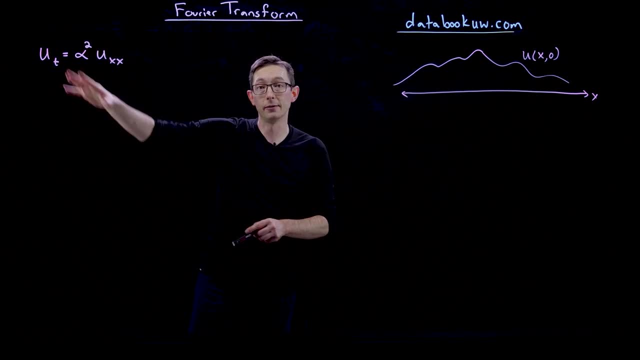 And this is my governing equation, This is the heat equation, okay, And so what we're going to do is we're going to Fourier transform this equation and we're going to show that it's very easy to solve this. This is a partial differential equation in space and time. 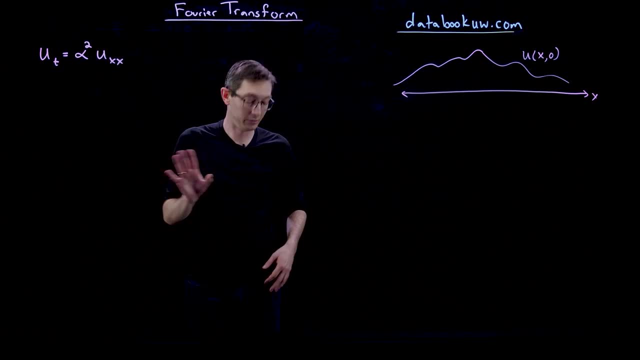 but when we Fourier transform, we're going to get a simple, ordinary differential equation out. okay, That's what I'm going to show you. So let's do this. and I just want to remind you that, remember, u is a function of x and t, and so if I Fourier transform this function of x and t, 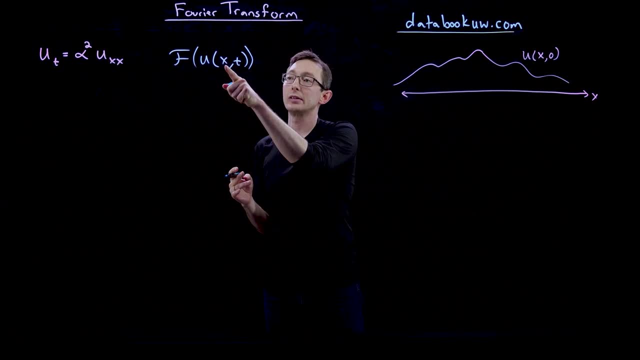 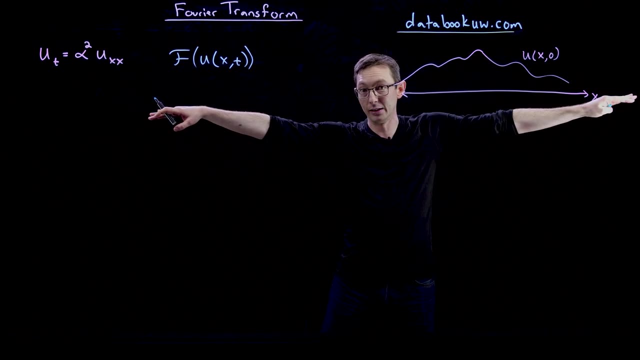 I'm Fourier transforming. I can choose space or time, but I'm going to Fourier transform with respect to space. okay, So space is my coordinate that goes to negative infinity and positive infinity. Usually we think of time as starting at zero and going to positive infinity, So space is kind of a two-sided infinite. 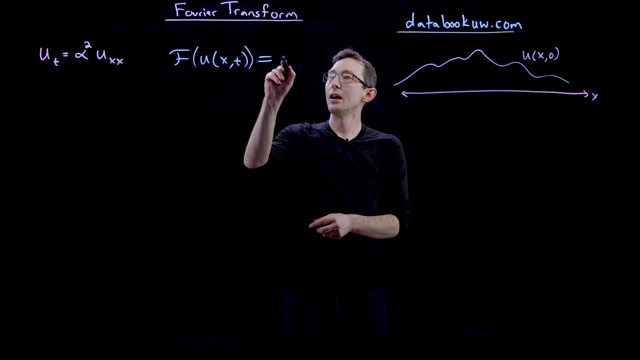 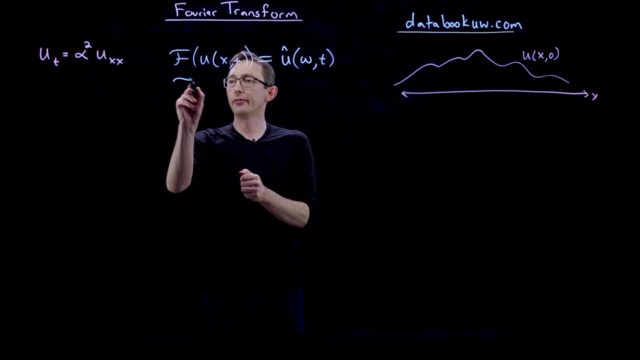 variable And so if I Fourier, transform with respect to space, I'm going to get this u-hat of omega and t, Good, okay, And of course, remember that the derivative of u with respect to x. if I take f of ux, so ddx of u, then I'll get an i omega u-hat, And if I take f of uxx, 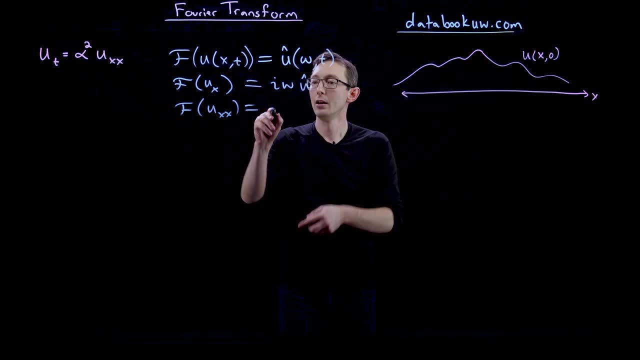 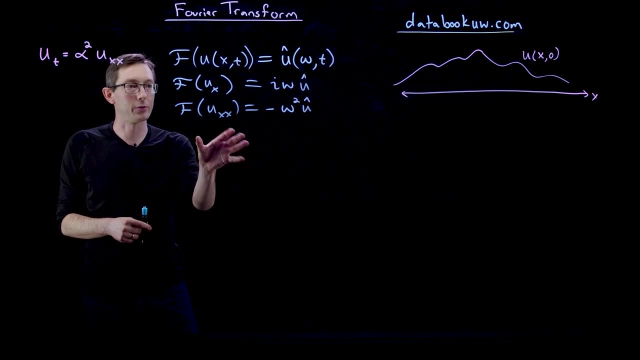 I'll get two i omegas out. I'll get an i omega squared which is a minus omega squared. u-hat, Okay, good. So that's that nice property of the Fourier transform, that the Fourier transform of derivatives is just i omega times, that Fourier transform Good. 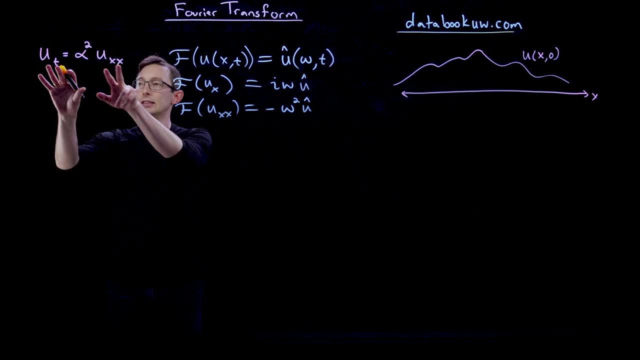 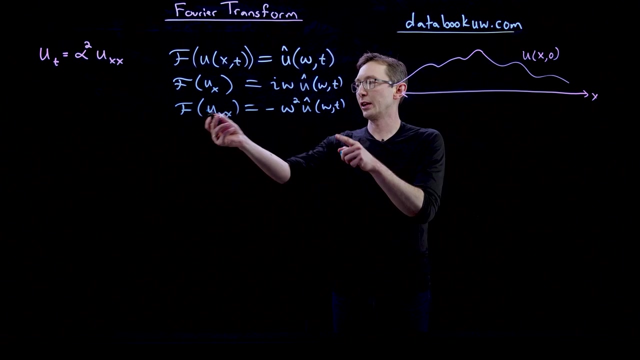 So now what we're going to do is we're going to transform this pde in u using these Fourier transform rules. okay, And maybe I'll be super explicit: This u-hat is still a function of omega and t, So my time variable didn't change, Remember. I'm just Fourier transforming with. 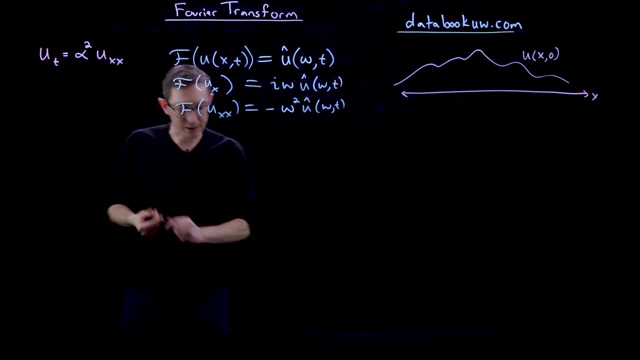 respect to space. okay, So that's what we're going to do. We're going to Fourier transform this with respect to space. So we're going to Fourier transform And what we're going to get is ddt of u-hat equals. now the Fourier transform of uxx is just minus omega squared u-hat. 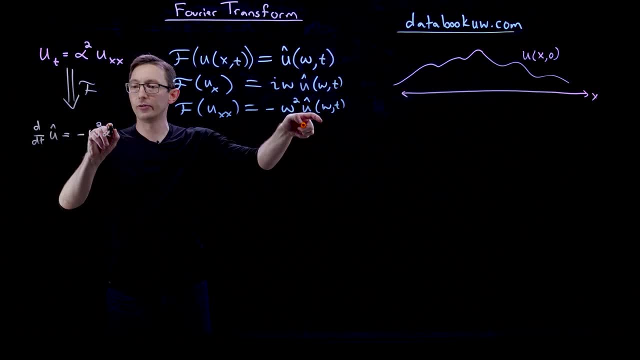 So I'm going to have a minus omega squared, alpha squared, u-hat Good, And this is really nice. This is a function of omega and t. And this is a function of omega and t. This is no longer a partial differential equation. This is just an ordinary differential equation with a time derivative. 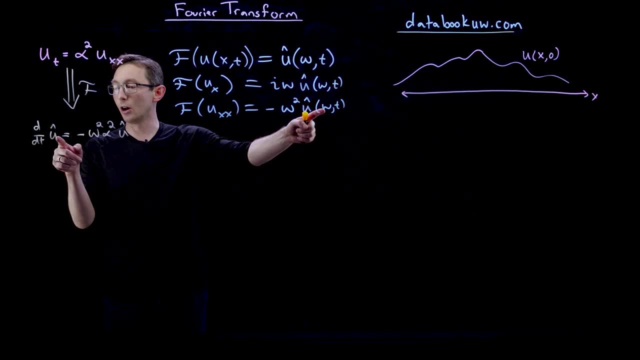 time derivative equals some function and for each Omega, if I lock in Omega, this is just a function of time and it's a normal, ordinary differential equation in time for each fixed Omega. okay, that's the key here. so now what we're gonna do is we're going to solve this ODE in time. that's actually quite simple, so I can. 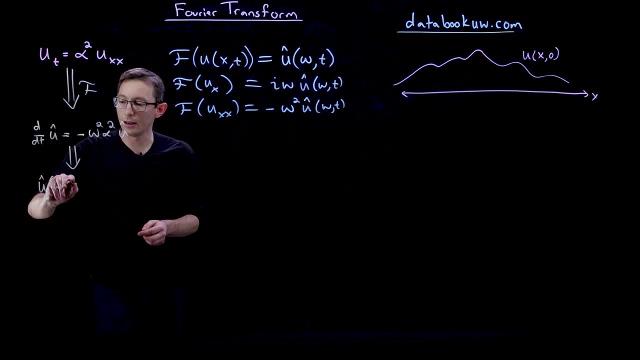 say that u-hat of Omega at some future time. T is just e to the minus Omega squared alpha squared T times u-hat of Omega at an initial time? T not, this is just how you solve an ODE- you at some time. T is e to the lambda: T times u at. 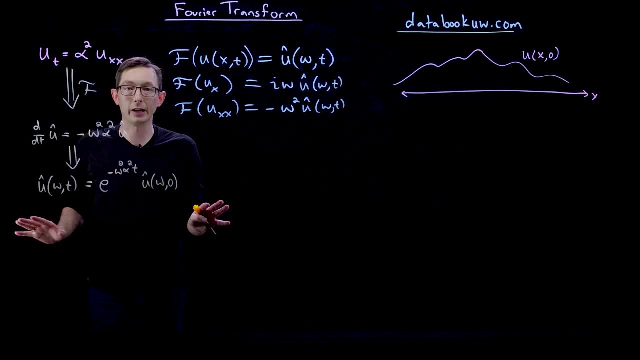 time, not at time, zero. okay, this is just the normal way of solving an ODE, and just think about how much simpler this is, the solution solving the full PDE right. you could use I don't know some PDE method to solve this, but by Fourier transforming we just get an ODE for. 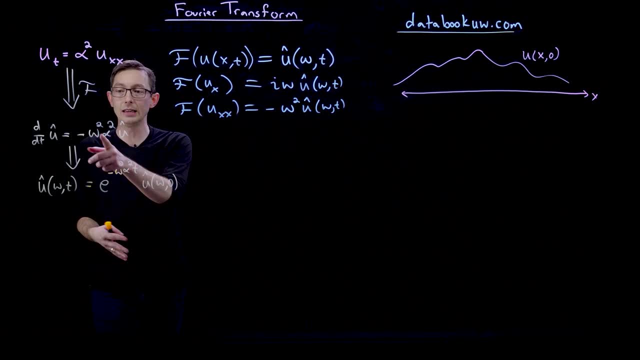 every fixed value of Omega. so we get a family of ODEs for every Omega, and this is the solution. okay, now, this is kind of cool. this is a Gaussian function. okay, this is a maybe I'll I'll change my colors a little bit. so this is a Gaussian. 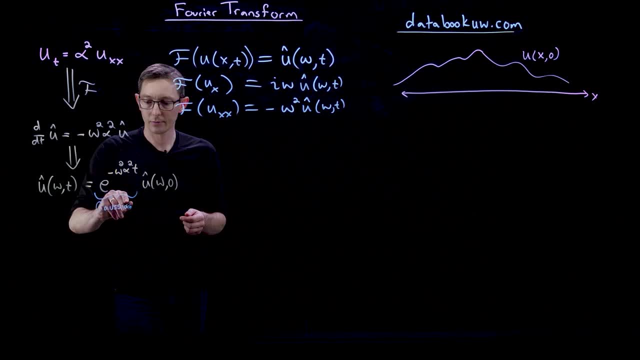 kernel, a Gaussian, and essentially what we can do. this is the product u-hat at Omega and T is the product of two functions of Omega. okay, so this is like F? hat and G hat and remember, if we inverse, Fourier, transform F hat times G hat, the inverse. 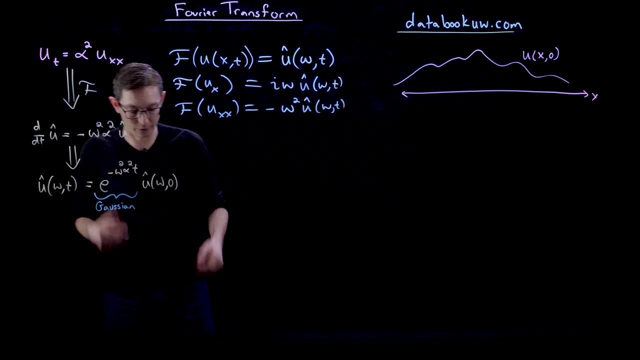 Fourier transform is just the convolution of the two inverse Fourier transforms. okay, and that's what we're gonna do now. so what we actually want, we don't want the solution in Fourier coordinates, we want the solution in in physical coordinates. we want to know what the final time heat distribution is, and so what we're going to do is we're going to 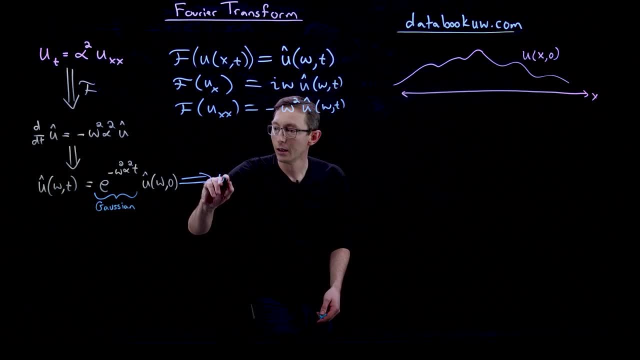 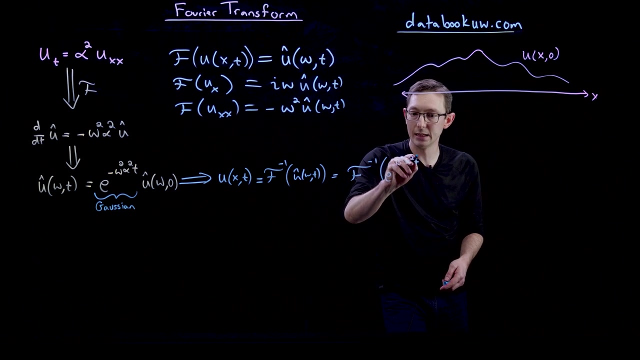 map back to original coordinates. we're going to say: u of X and T is equal to the inverse Fourier transform of u-hat Omega and T, which is going to be equal to the inverse Fourier transform of this Gaussian, this e to the minus Omega squared Alpha squared T. convolution integral with the. 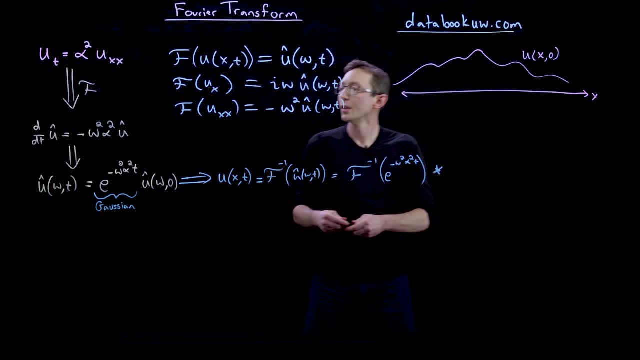 inverse Fourier transform of u-hat Omega not. but this u-hat Omega not is just the Fourier transform of my initial temperature distribution. so the inverse Fourier transform of this initial temperature distribution in for a coordinates is just my initial temperature distribution in regular space coordinates. so a convolution with u of X and T is one of those more common. even case when we first did the 11th intrigue for defense and just having a really complicated way of knowing anything else all gives you funny answers at all here. so let's try to see how we can use that. that's what I'm, because that's what we're. 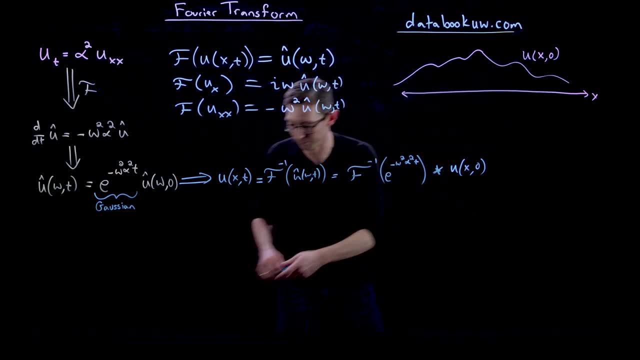 engineering wonder twist, and I use that merciful freedom test. so i'll start by x at time 0, my initial condition, And here's where it gets kind of interesting. So the inverse Fourier transform of a Gaussian is another Gaussian. That's a property you can derive using the Fourier transform integral. 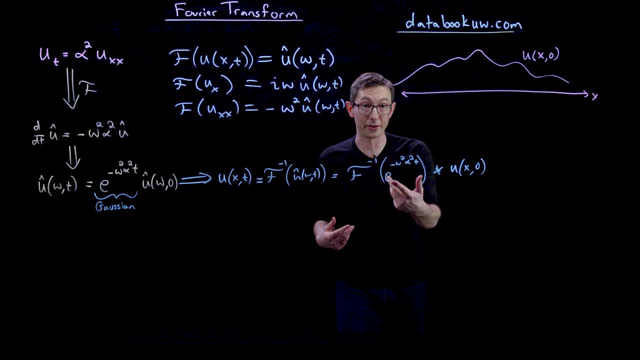 You can plug this in and show that your inverse Fourier transform is another Gaussian. So this is essentially another Gaussian in x and t. I'm just going to write a Gaussian in x and t convolution with my initial condition. my initial condition. And what's interesting is that, as time goes on again, 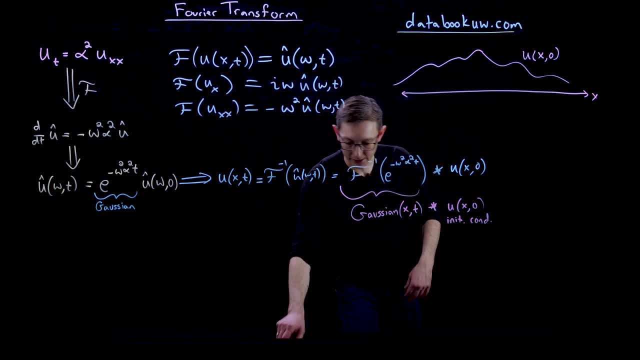 you'll have to work this out. I probably can actually write out roughly what this Gaussian looks like. This Gaussian is something like: 1 over 2 alpha square root of pi, t e to the minus x squared Over 4 alpha squared t, something like that. 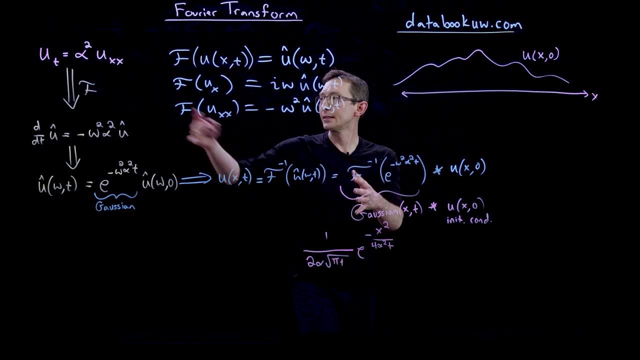 And so what this means is that, as time goes on, as time gets bigger and bigger, as time goes on with this initial condition, this Gaussian gets more and more and more spread out. So I'll just write this out. So I start out with a very, very sharp Gaussian. 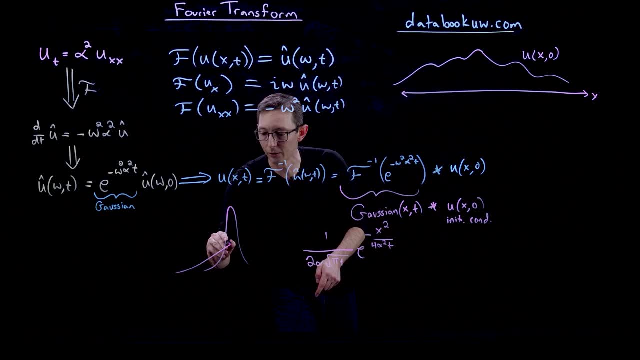 And as time goes on, this Gaussian spreads out and gets fatter and fatter and fatter And more and more diffuse. OK, so this is called a diffusion kernel, diffusion kernel, OK, And essentially what we're doing is we're taking our initial condition. 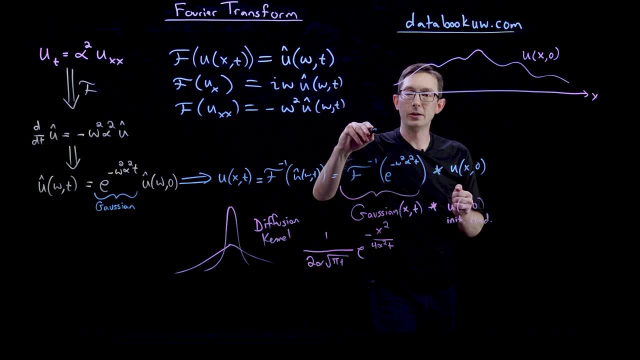 and we're convolving it with a diffusion kernel. So we take this diffusion kernel and we slide it across and take the dot product and we smooth out this distribution. It gets smoother and smoother and smoother And the more time passes, the wider it gets.